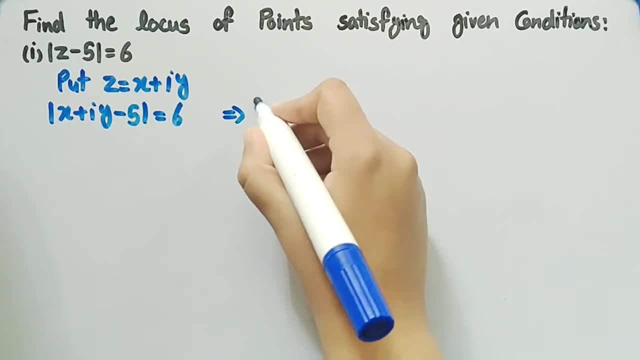 We can also write it as mod of x minus 5 plus iota y equal to 6.. Now, by taking the mod of this term, we get square root square of the real part of complex number, which is x minus 5, square plus square root of the real part of complex number. 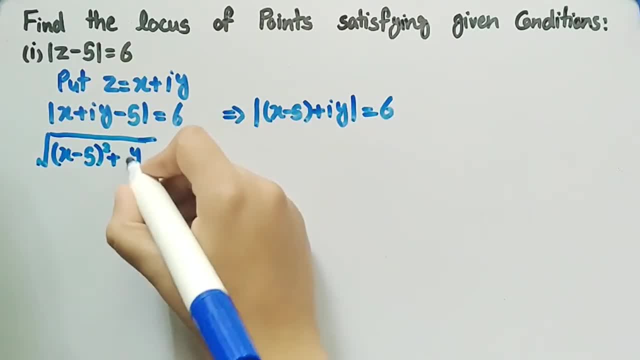 We can also write it as x minus 5 whole square plus y minus 0 whole square, equal to 6.. Now, by taking the mod of x minus 5 plus iota, y minus 5 square plus square root of the real part of complex number, which is x minus 5 square plus square root of the real part of complex number, 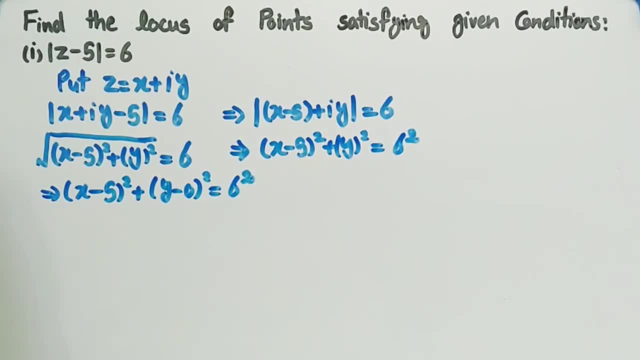 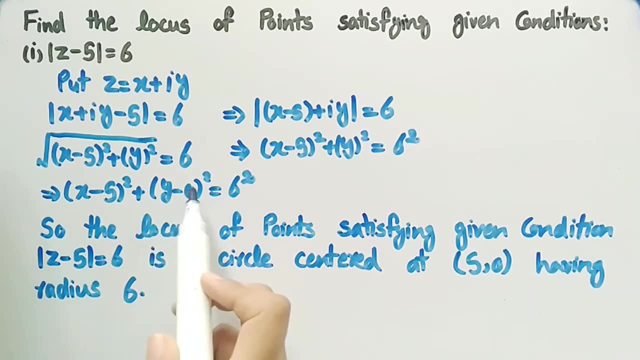 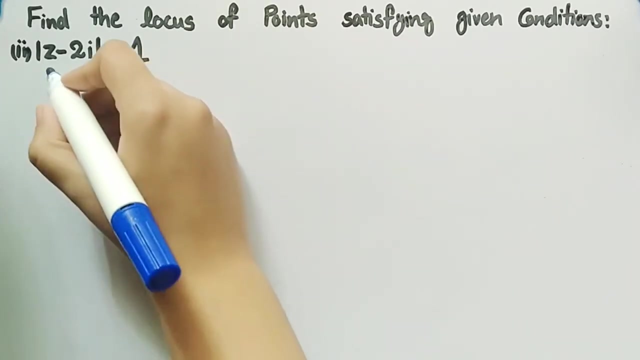 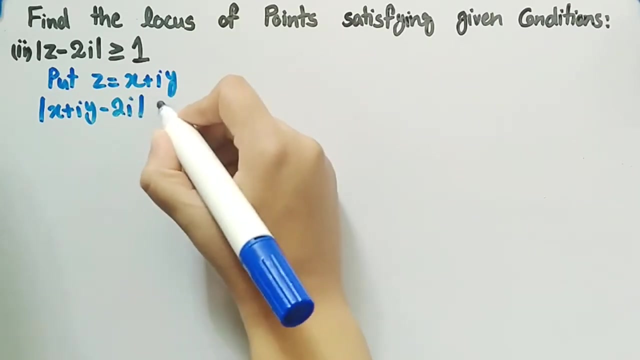 We can also write it as mod of x minus 5 plus iota y minus 5 plus square root of the real part of complex number, which is x minus 5 square plus square root of the real part of complex number. Firstly, we will put: z is equal to x plus iota y and we get mod of x plus iota y minus 2 iota greater than equal to 1.. 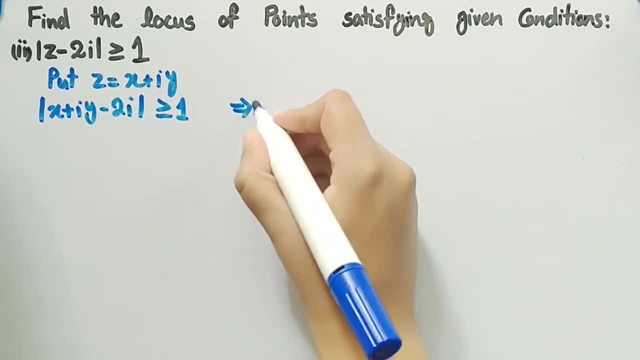 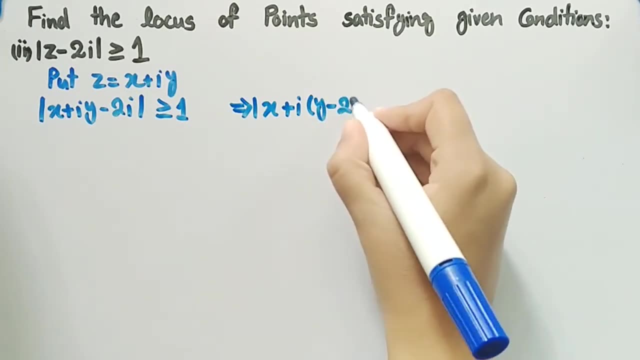 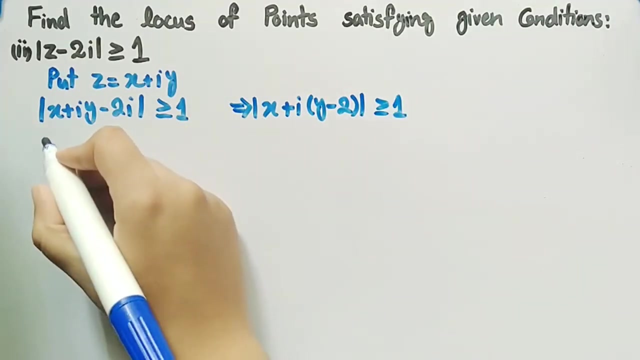 We can also rewrite it as mod of x plus iota into y minus 2 greater than equal. Now, taking the modulus of this complex number, we get square root square of real part, which is x, and we get x square plus square of imaginary part, which is y minus 2 square greater than equal to 1.. 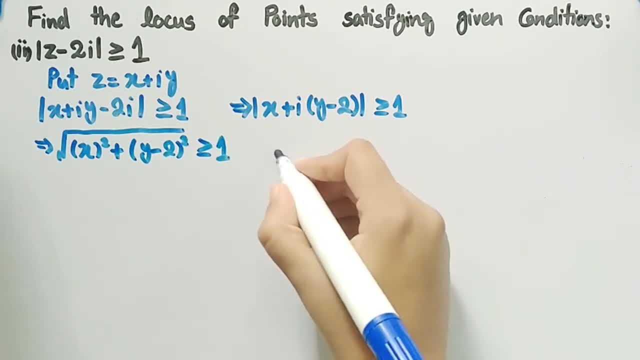 Now, by squaring both sides of this equation, we get x square. We can also write it as mod of y minus 5 plus y minus 2, whole square greater than equal to 1.. So we can see that this equation resembles the equation of a circle. 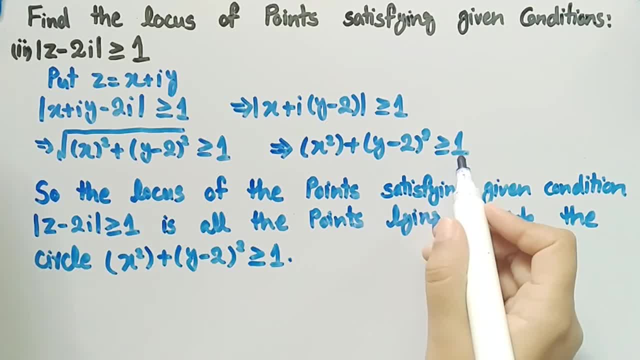 Since there is this greater than equal to 1 condition, so the locus of the point satisfying given condition mod of z minus 2 iota greater than equal to 1.. all the points lying outside the circle x square plus y minus 2, whole square. 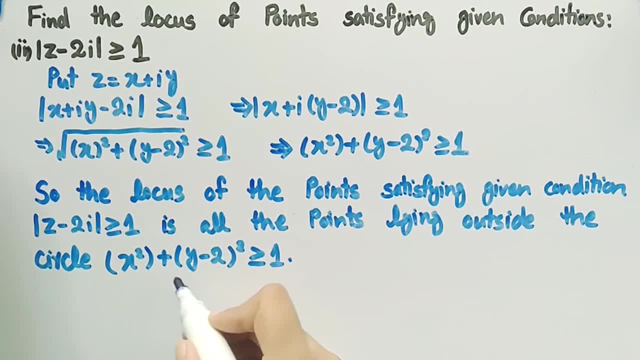 greater than equal to 1, since this locus satisfy this condition- greater than equal to 1- so all the points will be outside the circle. for example, if we suppose that this is the circle, then the locus will be all the points that will be on the boundary of the circle and outside the circle. the third one is: 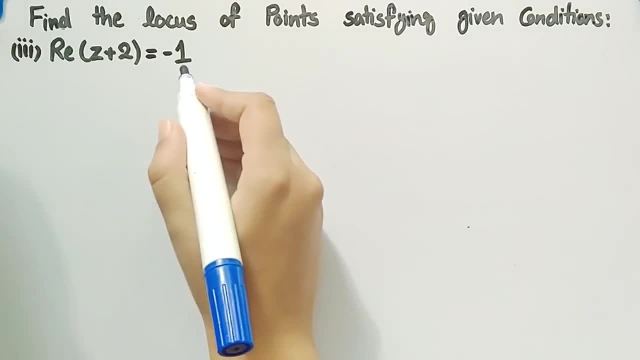 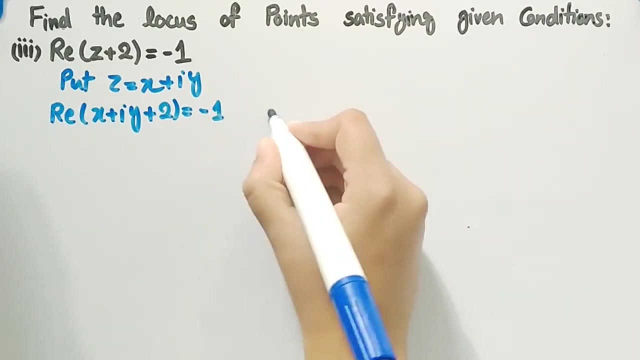 real of part of z plus 2 is equal to minus 1. so firstly we will put z is equal to x plus iota y in this equation and we get real part of x plus iota y plus 2 is equal to minus 1. we can also rewrite it as real part of: 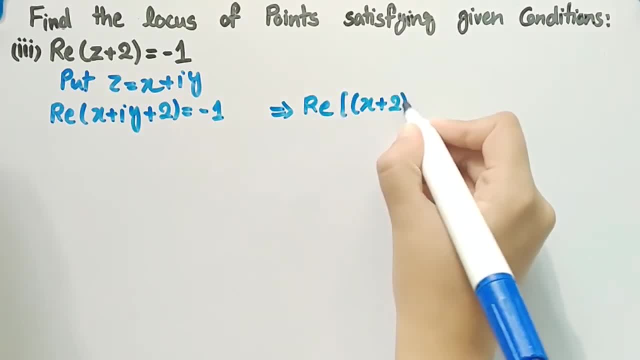 x plus iota y plus 2 is equal to minus 1. we can also rewrite it as real part of x plus iota y plus 2 is equal to minus 1. we can also rewrite it as real part of x plus 2 plus iota y, equal to minus 1.. Now we can see that the real part of this complex number. 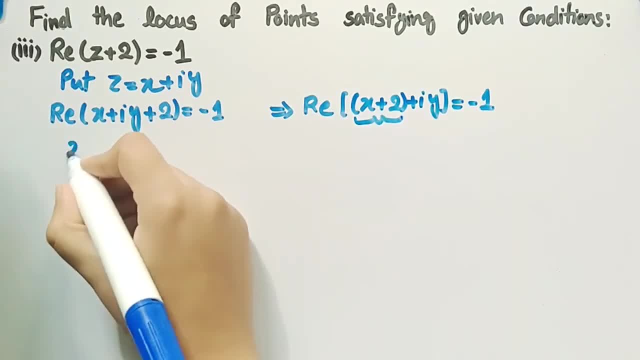 is x plus 2.. So we can write x plus 2 equal to minus 1.. Here we have just written x plus 2 because it is given that we have to write real part of this complex number, which is x plus 2.. 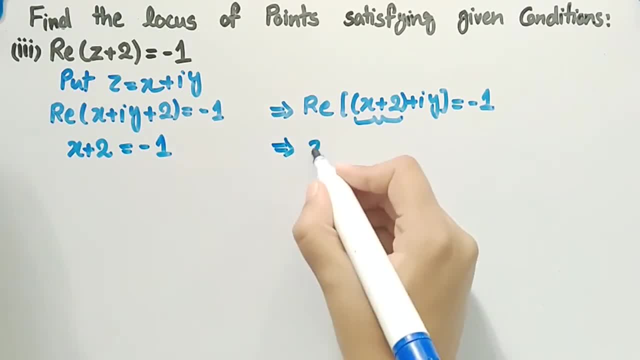 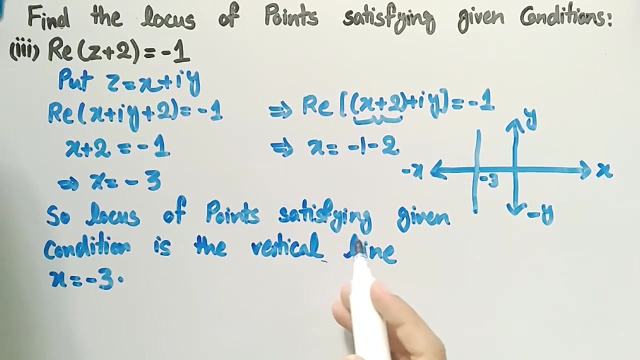 Which implies x is equal to minus 1 minus 2.. So x is equal to minus 3.. So the locus of point satisfying given condition is the vertical line. x is equal to minus 3.. We can also see its graph. Fourth: 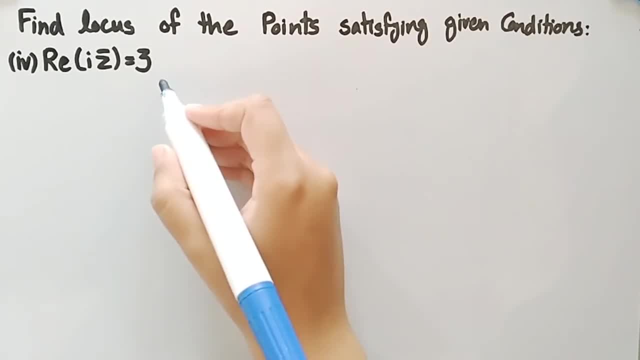 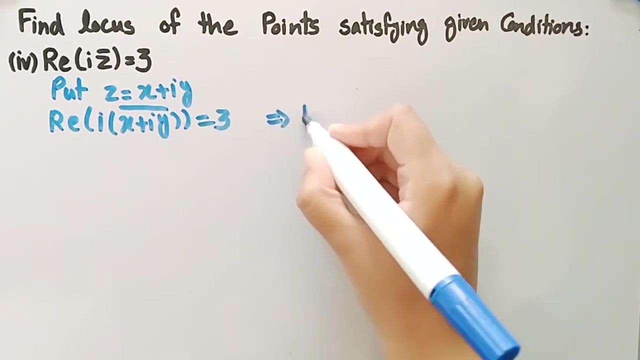 is real part of iota z conjugate is equal to 3.. Firstly, we will put z is equal to x plus iota y in this condition and we get real part of iota x plus iota y conjugate is equal to 3.. Which implies real part of iota x plus iota y conjugate is equal to 3.. 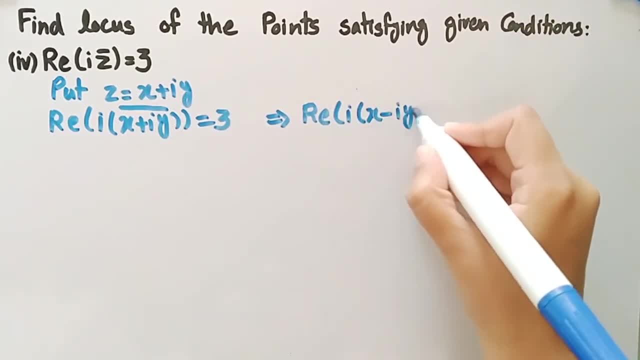 We can also write it as real part of: if we multiply iota, we get iota x minus iota square y equal to 3.. We can also write it as real part of: if we multiply iota, we get iota x minus iota cube y equal to 3.. 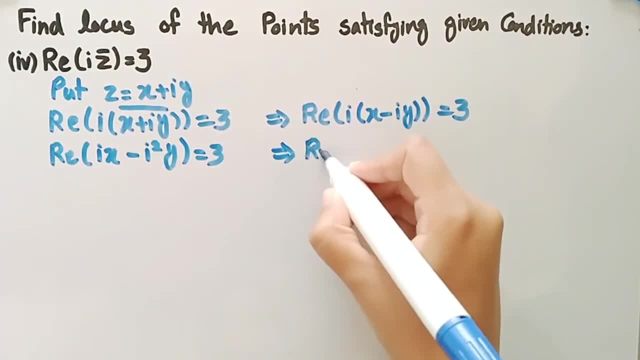 It can also be written as real part of iota x minus iota cube y, coordinate as iota square y近 3.. The there will be a run in of each iota whichắm is written as piece iota y. So if we vasoli this well, it will not work, And if we mess up, we get x plus 3 and hence it is less than. 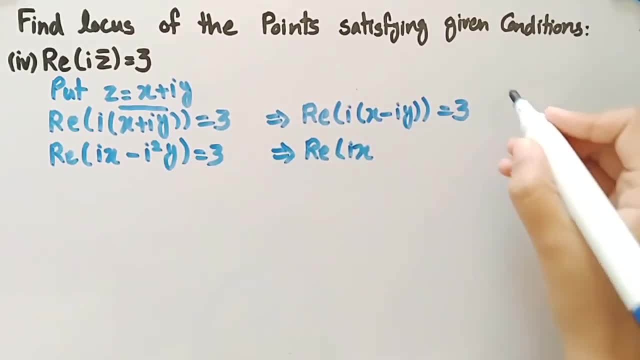 We can have 3 plus z, which is equal to 0.. So if we multiply by a, iota square will be equal to minus times. iota square is equal to minus 1, so it is equal to 1. so here we get plus y equal to 3. here we have to take the real part of this expression, which is y, so we can write it as: 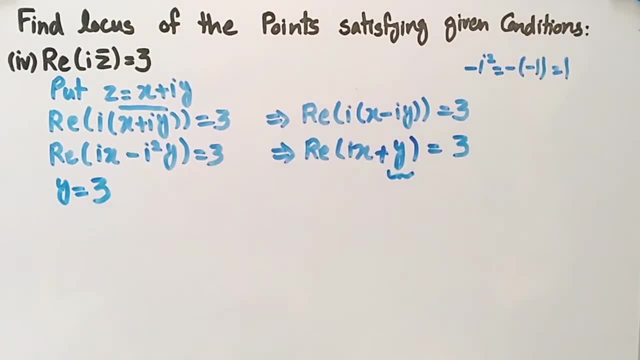 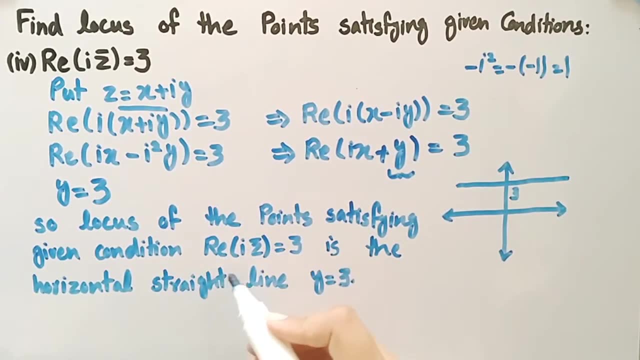 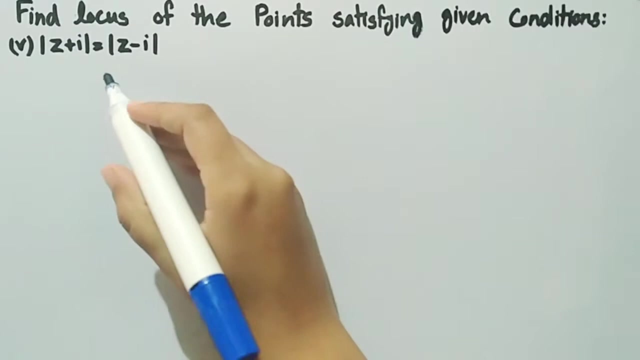 y is equal to 3. so the locus of the point satisfying given condition, real part of iota z conjugate equal to 3 is the horizontal straight line y is equal to 3. the fifth one is mod of z plus iota equal to mod of z minus iota. 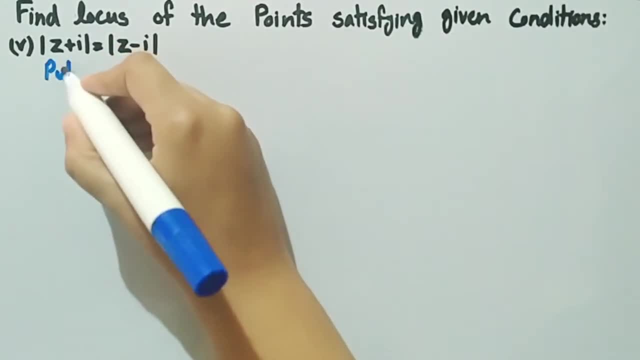 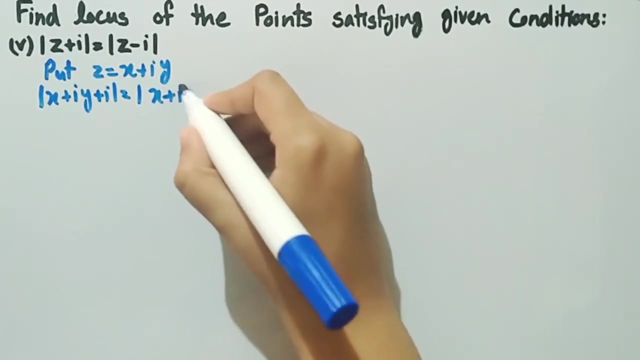 first we have to take the real part of this expression, which is y. firstly, we will put: z is equal to x plus iota, y, and we can write this condition as x plus iota, y plus iota, equal to mod of x plus iota, y minus iota. we can also rewrite it as: